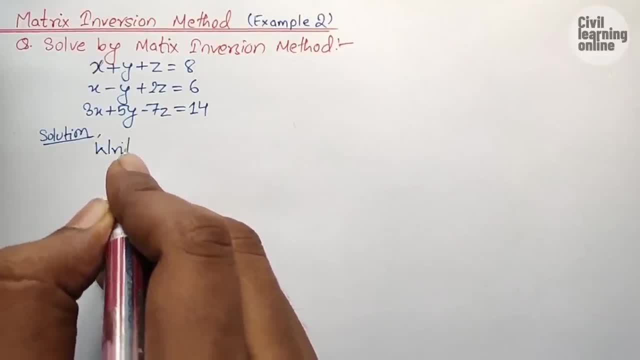 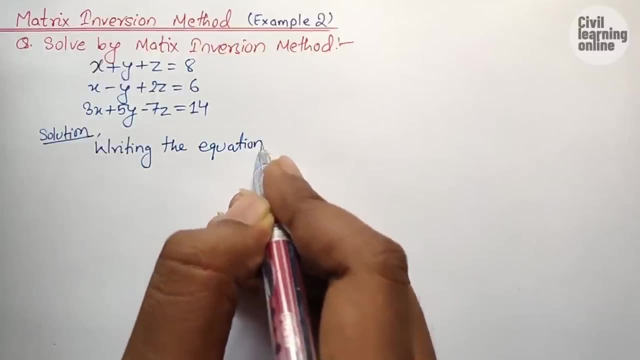 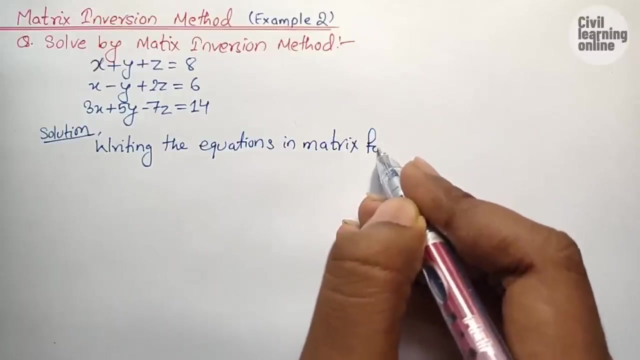 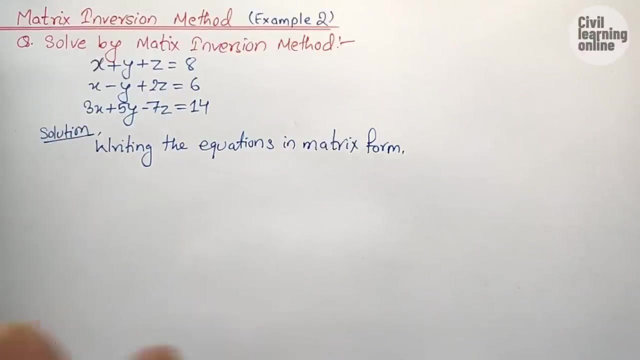 So write it down here, writing the equations, equations in matrix form. how we can write it in matrix form, let us see here: First we will separate the coefficient from each and every variables. so the coefficient of x here is 1, again here 1. coefficient of z is also 1 in first equation. similarly, the coefficient of x in second equation is 1 minus 1 and 2, 3, 5 and minus 7, 3, 5 and minus 7.. 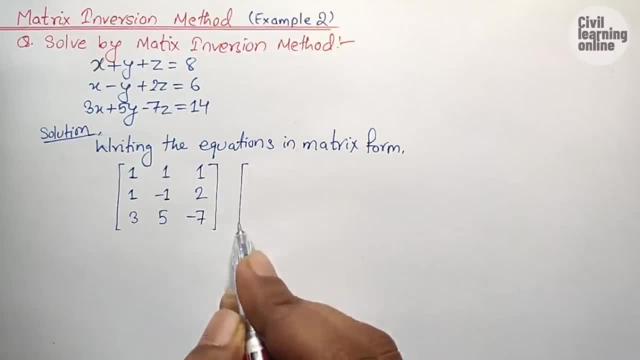 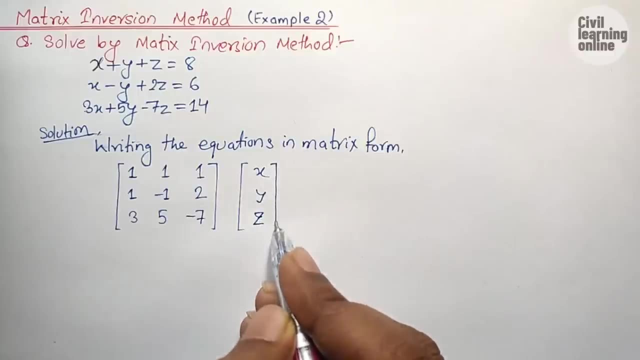 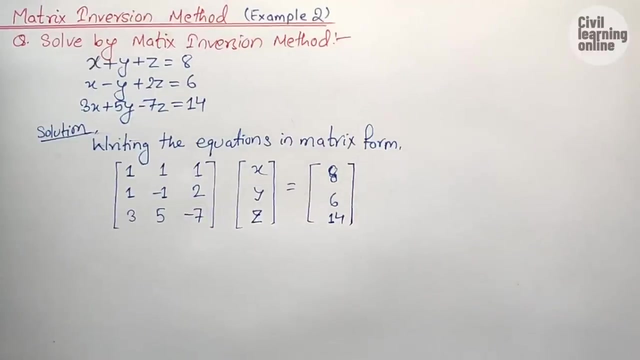 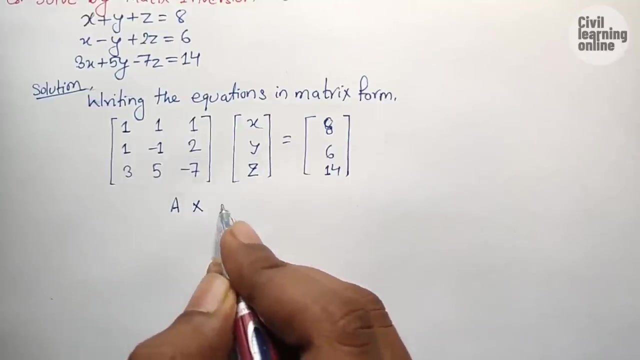 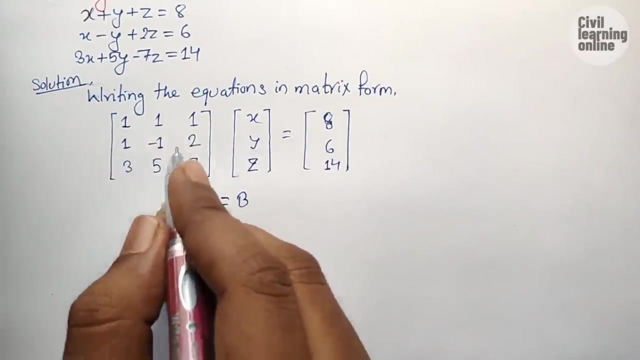 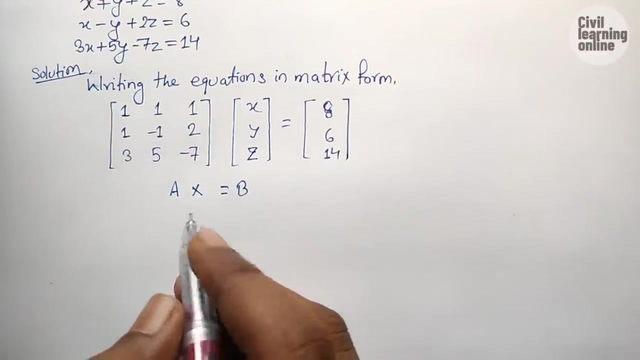 Now write all the variables in a single column. equals to sign and write down these terms, making a column 8, 6 and 14.. Now, guys, if I talk about the concept of matrix inversion, it says that a, x equals to b. here a represents this coefficient matrix, x represents these variables and b represent this column. now, guys, here, if we are asked to calculate the value of x, then x will be equals to a inverse b. here a is brought this side, so it will be b. 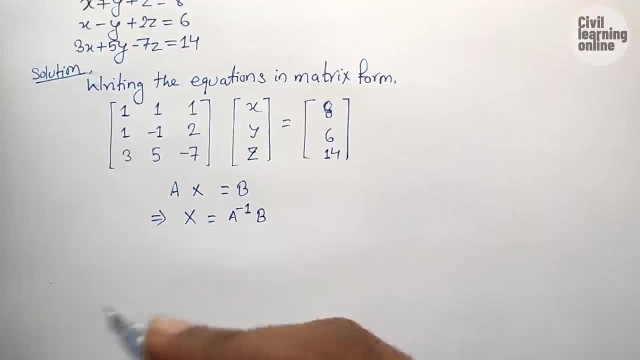 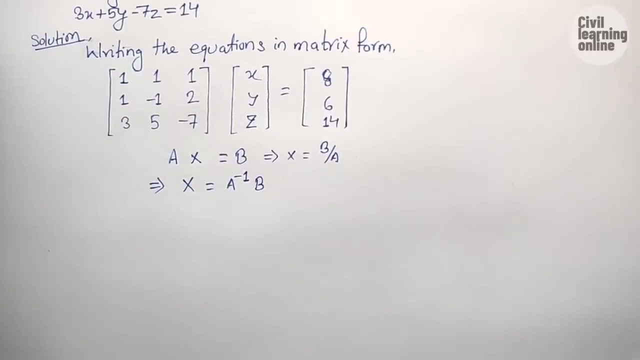 by a, and if I write a along with the b, then a will have the negative power. here what I said: x equals to b by a, and if a is brought with b, a is brought with b, then the power will be minus 1. I hope you know these things now. what we need to do is we have to calculate the inverse of a, and for calculation, 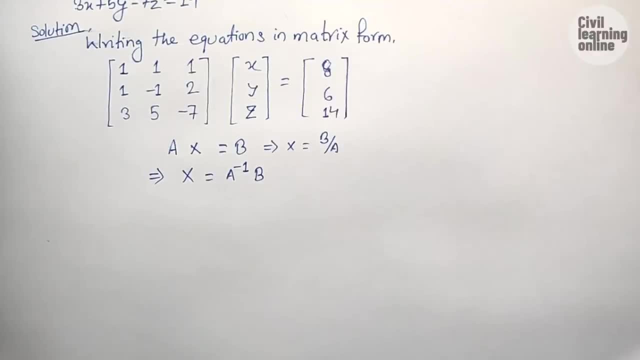 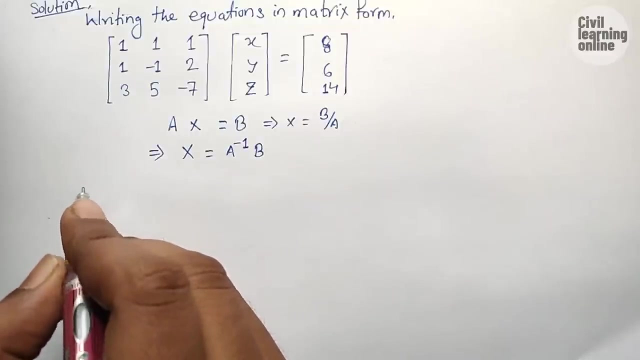 the inverse of a. first of all we need to find the determinant of a, and if our determinant is equal to 0 means its inverse does not exist. so let us first find the determinant of the matrix a and check whether it is equal to 0 or not. so if i calculate the inverse of matrix, sorry. 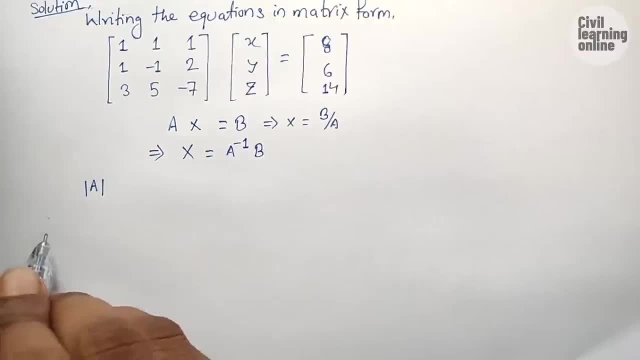 determinant of matrix a, then determinant is written by this form. so determinant of matrix and matrix a is 1, 1, 3, 1 minus 1, 5, 1, 2 minus 7, and if i calculate its determinant, then let us calculate the determinant using the first row. 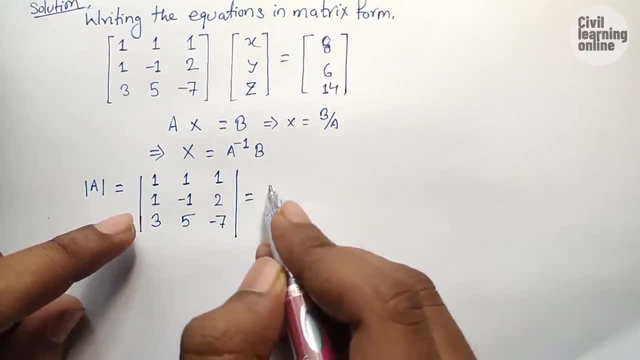 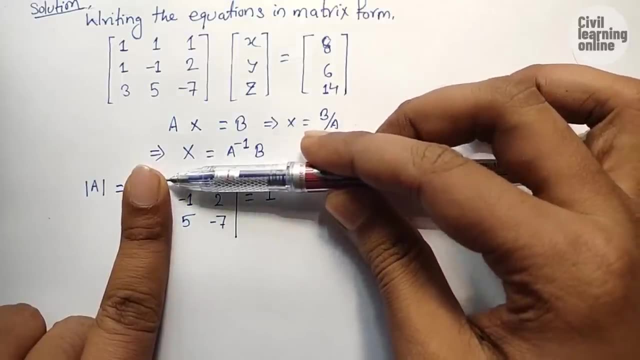 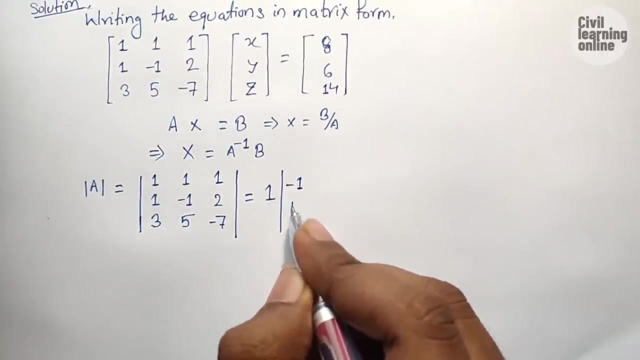 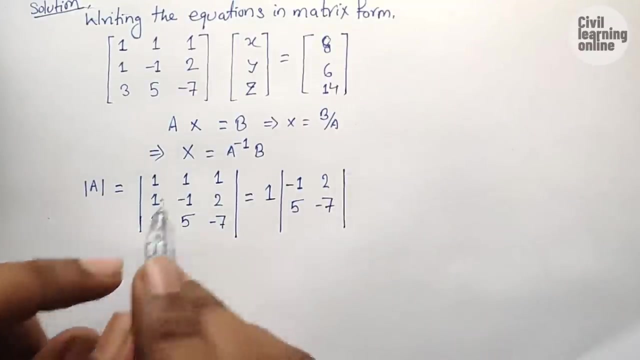 first row, then first row. if i select this one, then cover this, and this then remaining is minus 1, 5, 2 and minus 7. write it here: minus 1, 5, 2 and minus 7. similarly, if i talk about the sign of the matrices, then what is here? let me. 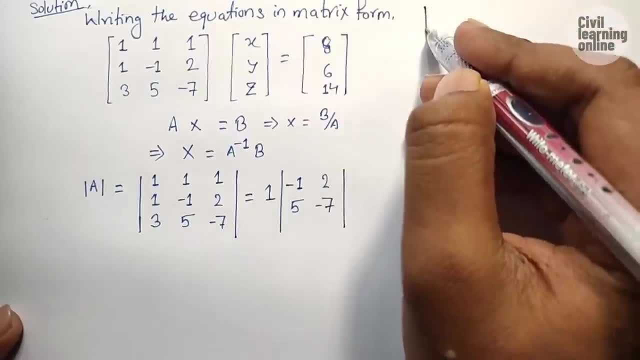 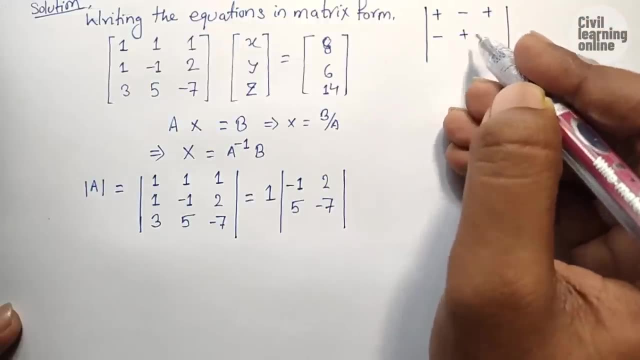 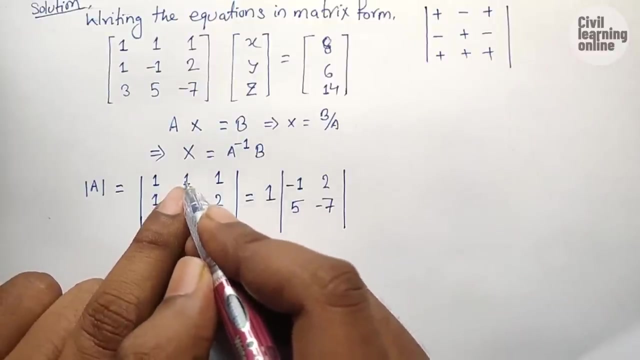 show you. let me show you here: the sign of the mat element of the matrix is equal to 0 and if i calculate the second row, then if i calculate, the second row of the matrix is equal to 0, and if i calculate the second row, then what it will have? then there will be negative. so now you will get to know a. 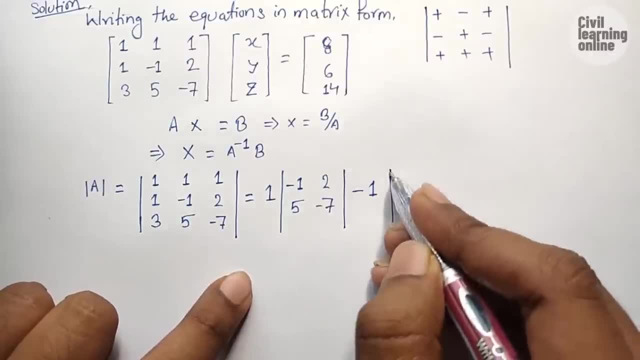 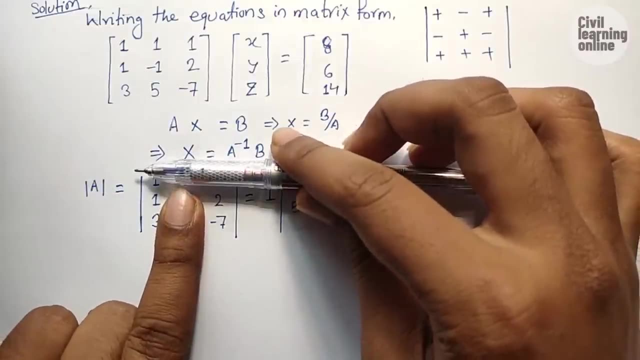 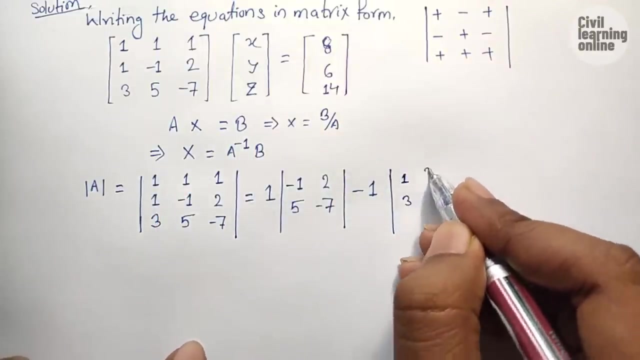 positive and negative matrix. the 204th matrix will be: i cannot use squander any way any following reasons: because we have never used and we have never knows лишuzas persona, alpha, negative, negative and items are 1, 3, 2 and minus 7. so 1, 3, 2 and minus 7 put positive sign this positive. 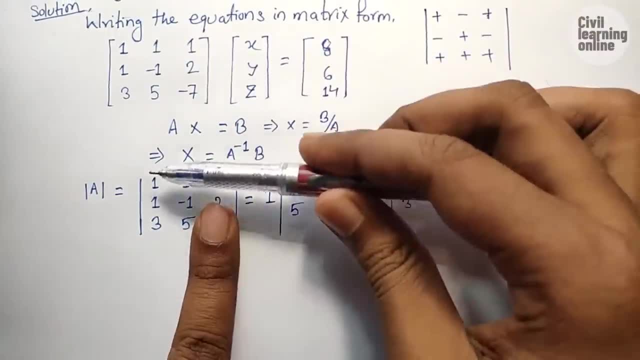 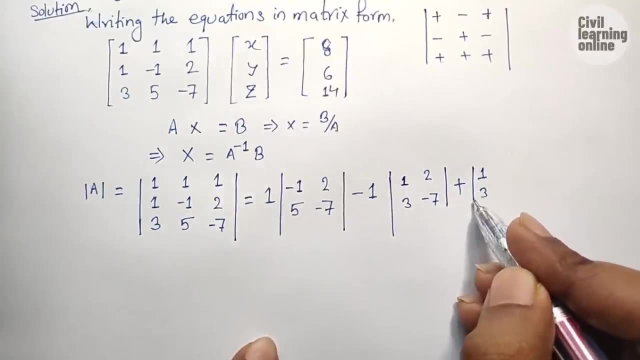 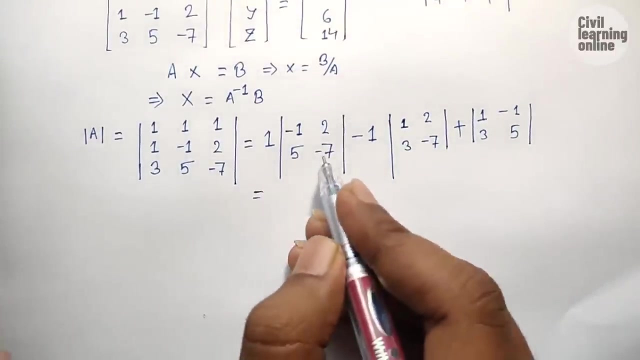 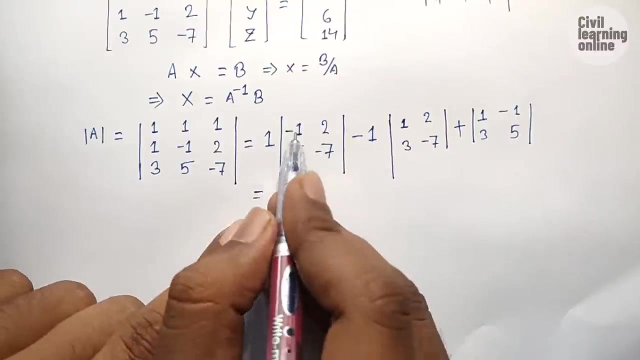 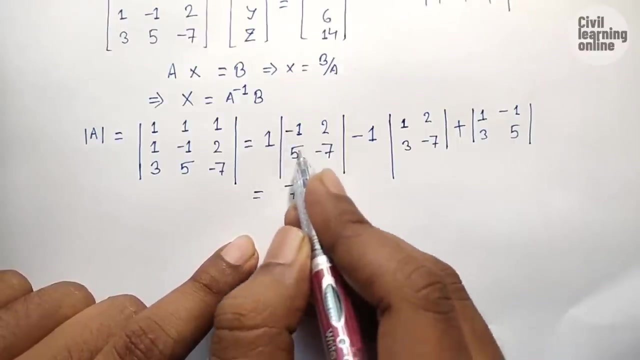 sign. so cover this and this. then we have 1, 3 minus 1, 5, 1, 3 minus 1 and 5. now solve this. we will have here 7 minus 10, what we do downward positive, upward negative. so downward positive means 7 times 1 will be 7 and minus times minus will become positive, 7 and 5 times. 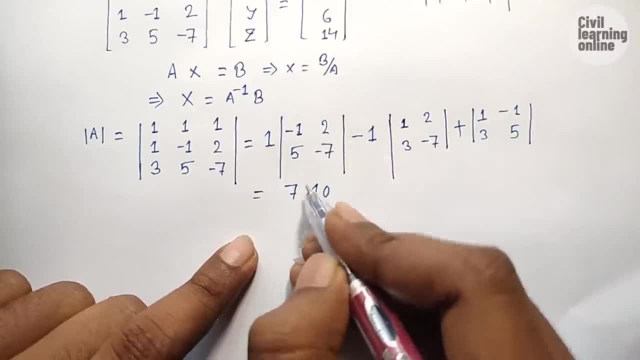 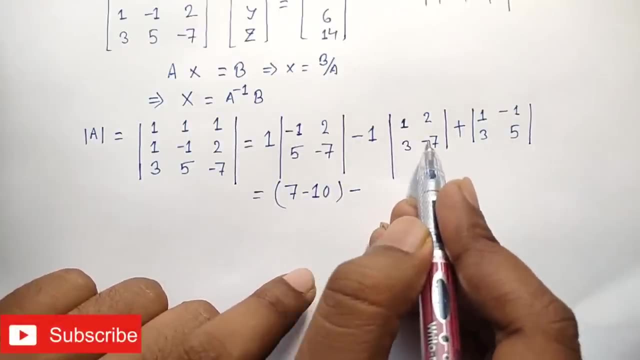 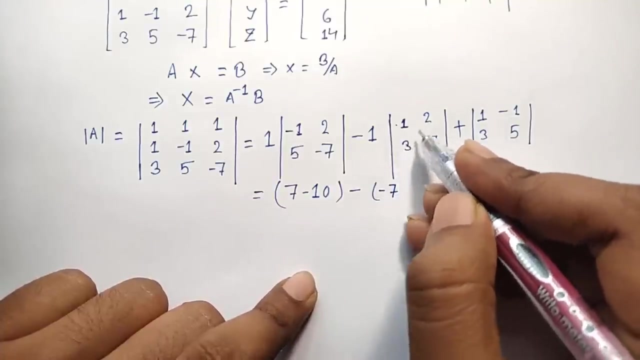 2 will be 10, but moving upward sign will be changed, so minus 10. now put this minus 1 here. minus 7 times 1 will be 7 and plus minus will be minus 7. again, 3 times 2 will be 6 and moving upward sign changed, positive will be written. 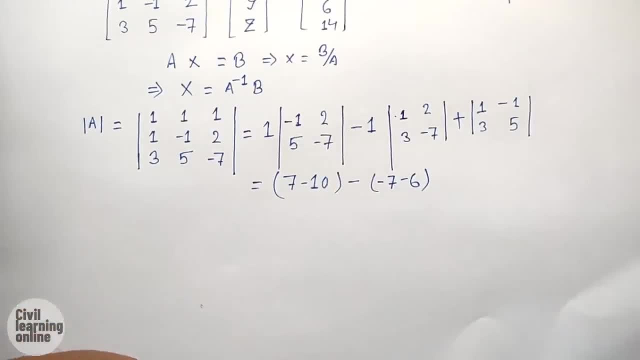 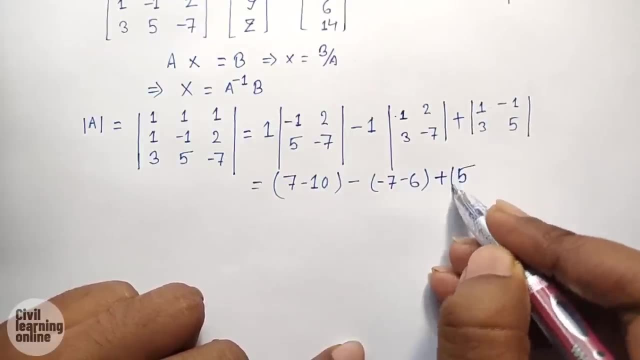 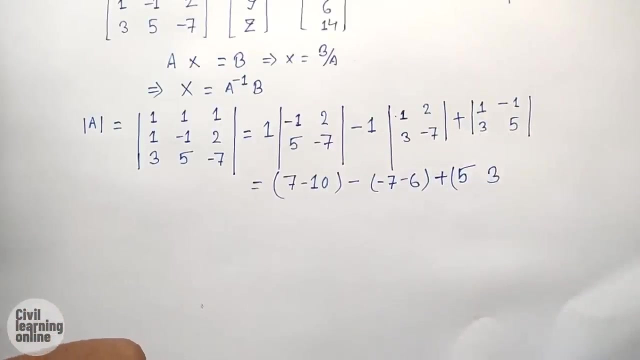 as negative. negative will be written as positive. actually it is multiplied with negative sign, so positive 5 times 1 will be 5 and 3 times 1 will be 3, and here minus times plus will be equals to minus. but on moving upward, sign is changed, so it will. 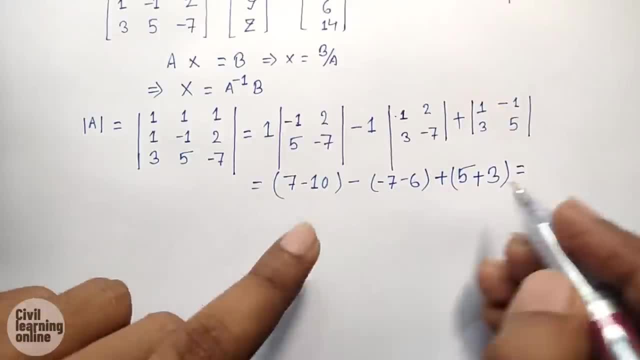 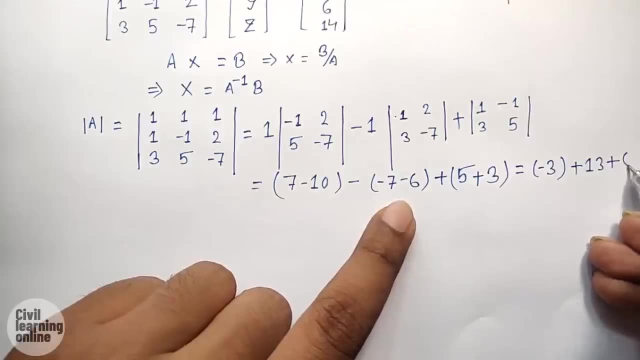 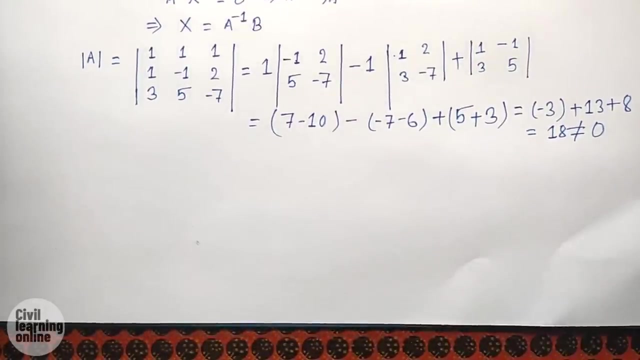 be positive. now solve this. we will get minus 3 plus 13 plus 8, and here it will be equals to 18, which is not equals to 0, means the inverse of the matrix a exists. now what we need to do is we need to find the cofactor of the matrix a. for that, let us see how to find the. 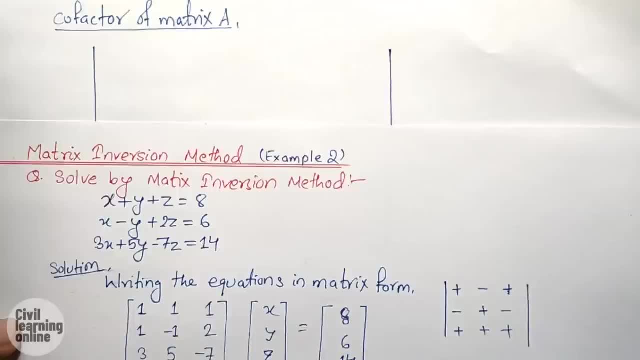 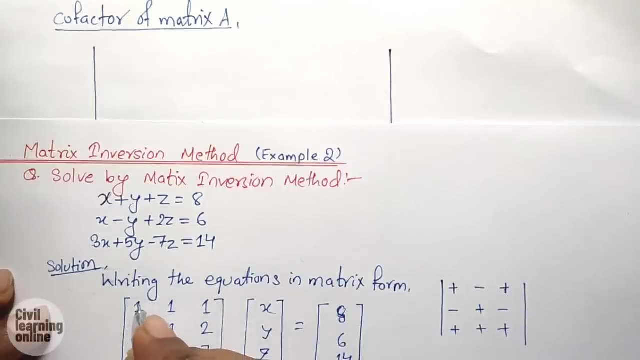 cofactor of matrix a. now see here, guys, how to find the cofactor of the matrix a. suppose we are. we need to. we are finding the cofactor of matrix of the element a 1: 1. this element is our a 1: 1. this. 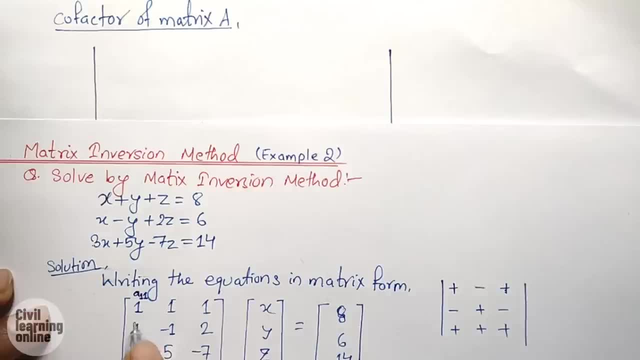 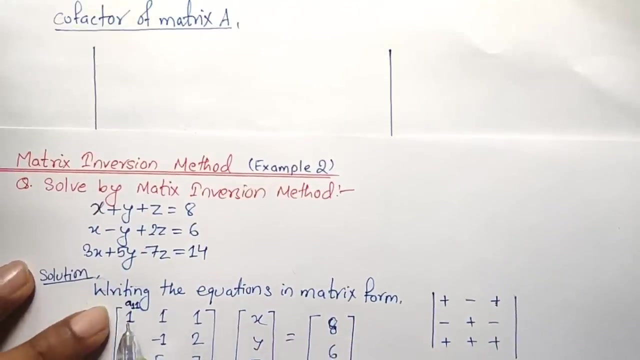 is a 1- 2. this is a 1- 3. similarly, this is a 2. 1 a 2. 2 a 2, 3 a 3. 1 a 3, 2 a 3, 3. this is actually the numbering of the element of the matrices. so if i select, find the cofactor. 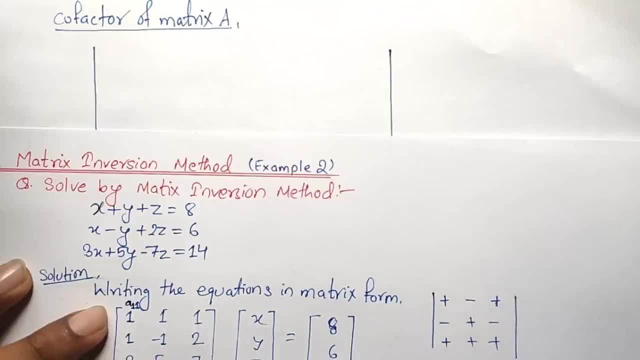 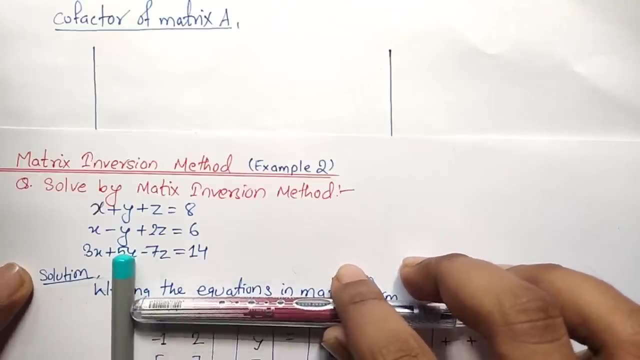 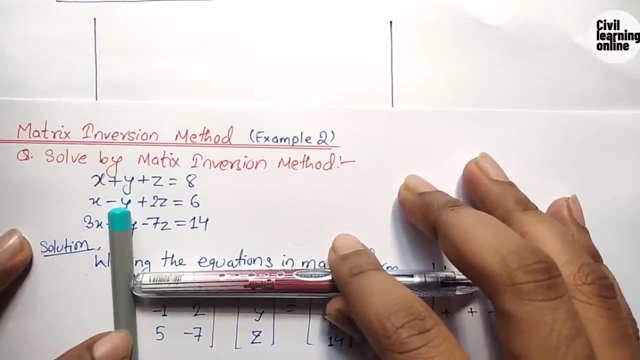 of this matrix, of this element 1 a, 1, 1, then what we need to do is simply cover this and cover this and write down all the elements which are visible to you. you, the number which are visible to you, are minus 1, 2, 5 and minus 7, so write it here. 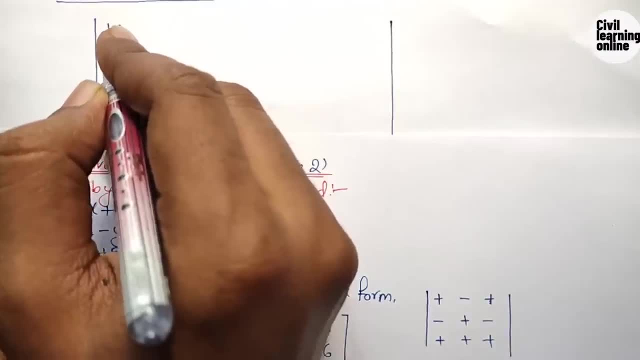 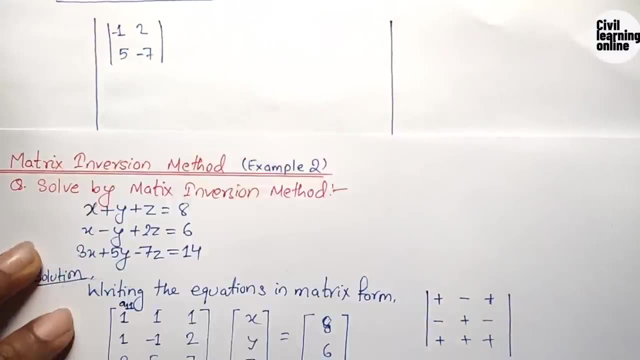 you minus 1, 2, 5 and minus 7. similarly, here the sign convention which i have shown you is positive, so write, put it here. positive sign for a 2- 1. this element is our a 2, 1, sorry. a 1, 2. first row, second column: a 1- 2. so the element of the element of 2 is plus. 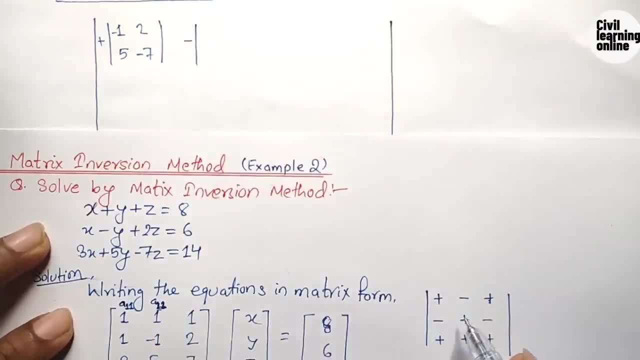 or equal to 1, so the element of the element of the table 1 value of a 2 is equal to a 2. clipping chair bridge bridge area. for any previous class we need. the column of the table of the first row, second column carries negative signs, so put here negative sign. 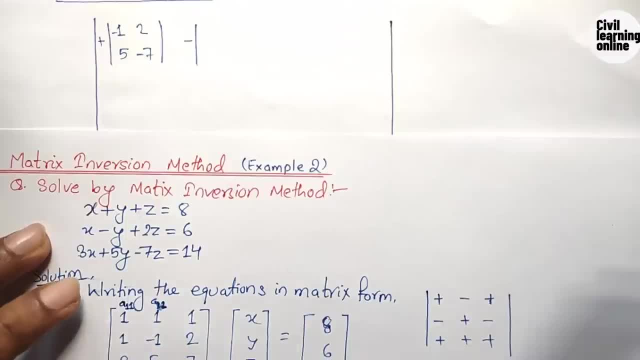 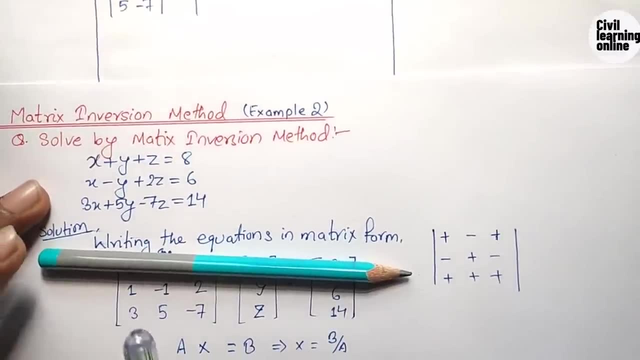 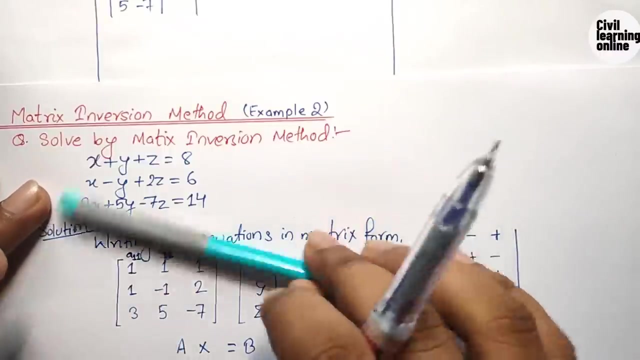 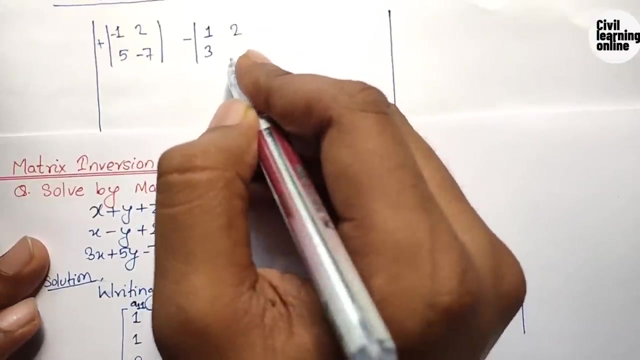 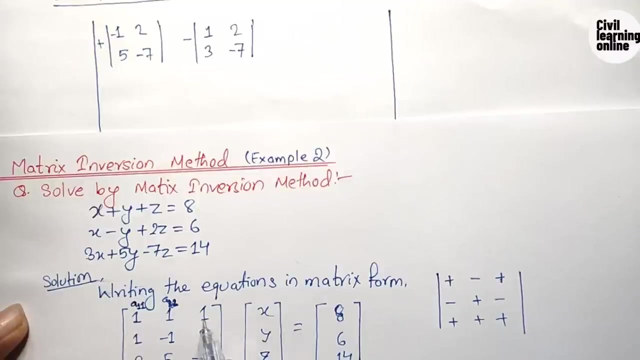 and cover the all the row and column which includes this element. so, on doing so, we will have here. let me show you here, on doing so, what we will have here. the element which will be visible are 1, 3, 2 and minus 7. write it here: 1, 3, 2 and minus 7. so now, if we talk about the element, 1, 3. 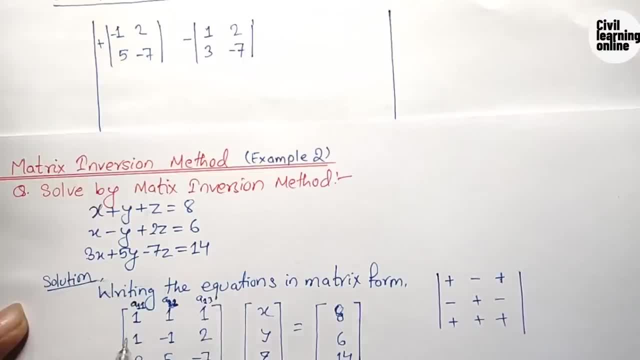 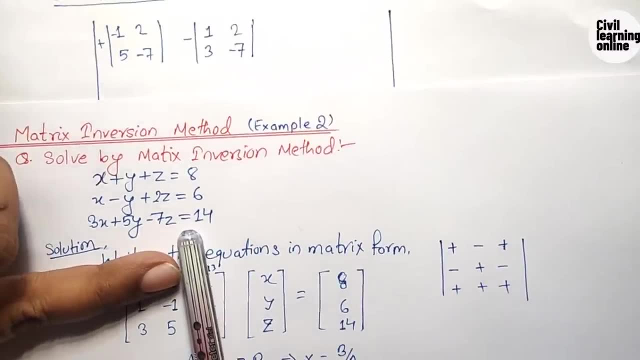 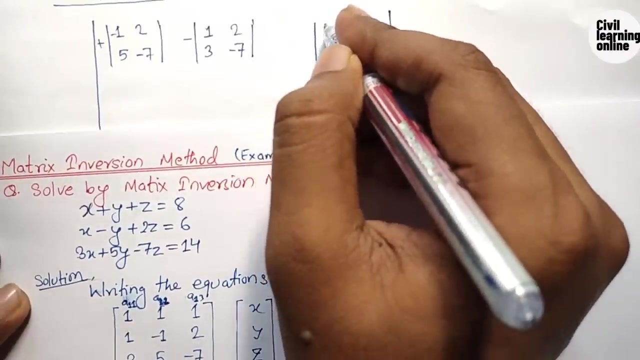 a 1: 3, first row, third column, then cover this and this, the element which will be visible to you, are 1, 3 minus 1 and 5. so 1, 3 minus 1, 3 minus 1 and 5. so here we need to write 1, 3 minus 1 and 5, the sign which it carries. 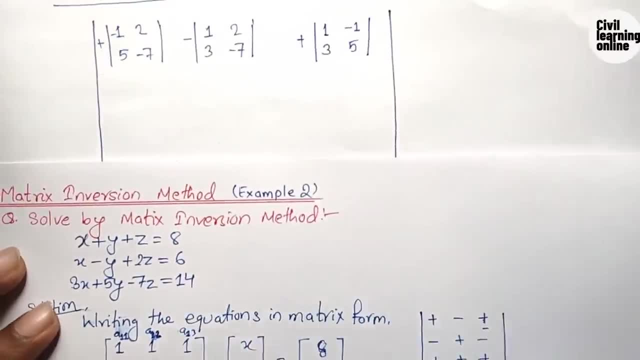 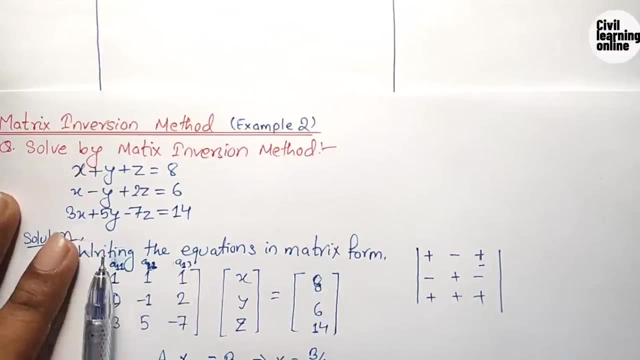 is positive. positive. now move here. move to the element of a: 2. 1 means second row, first column, this one. so what we need to do is we need to cover all the row and column which carries, which consists of this element. so the number which are visible. 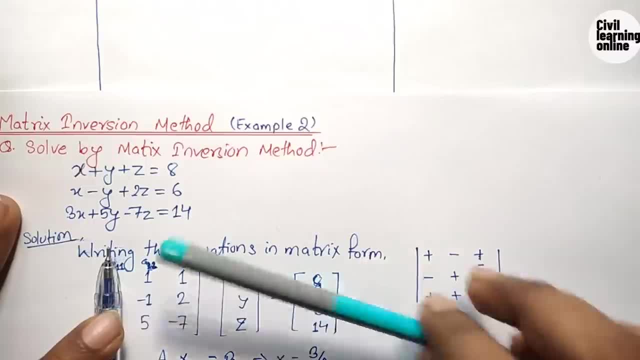 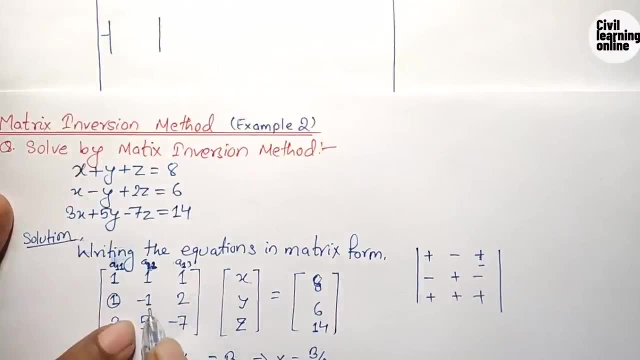 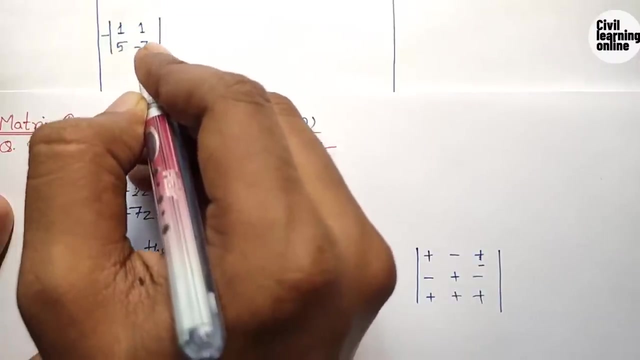 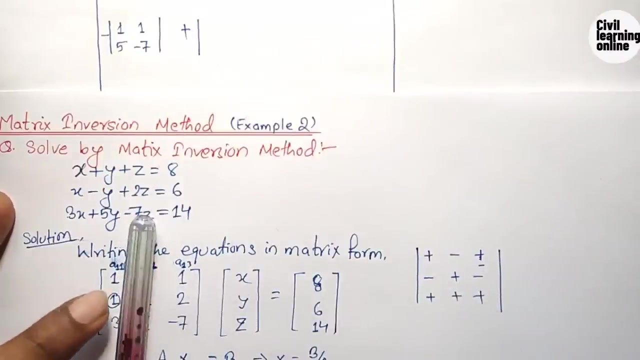 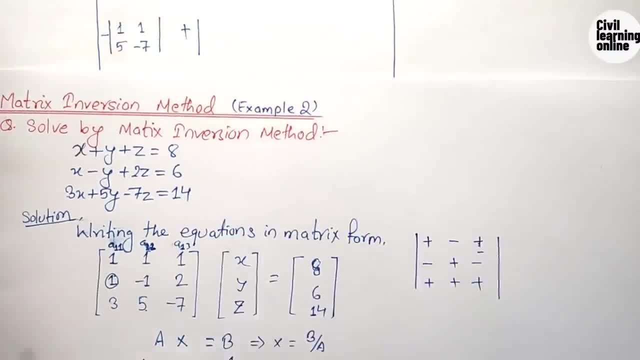 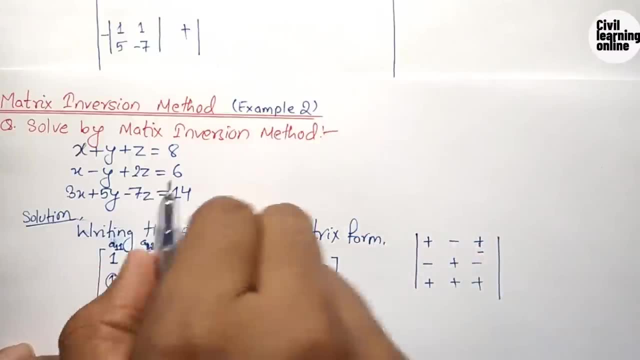 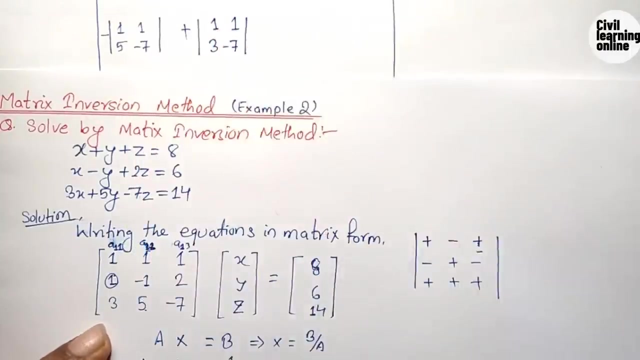 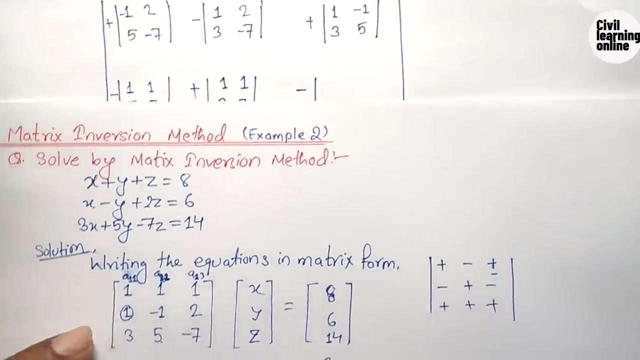 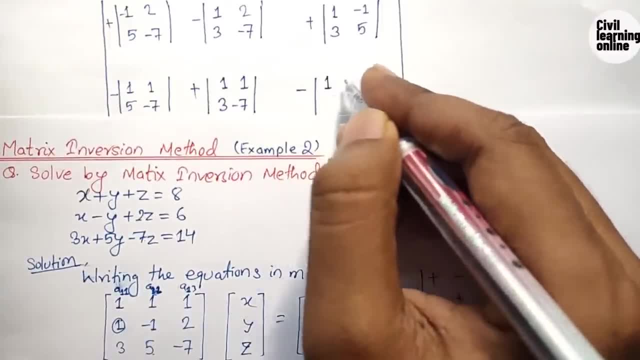 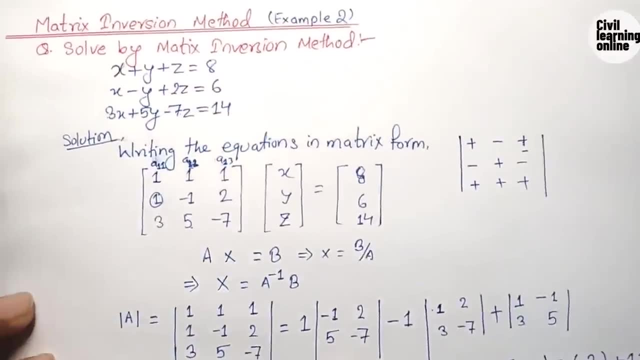 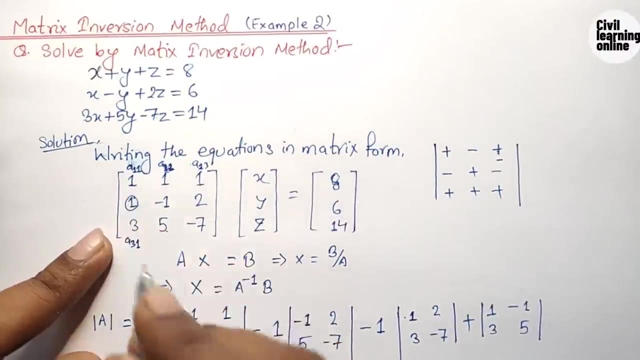 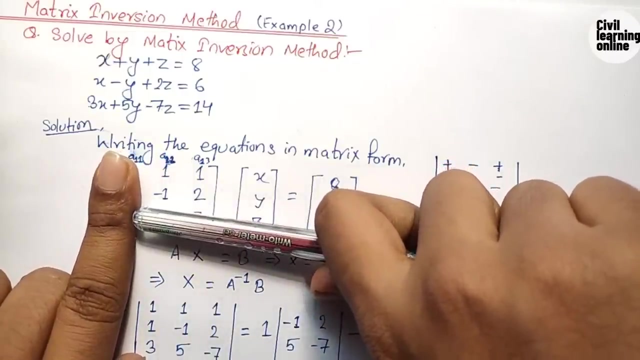 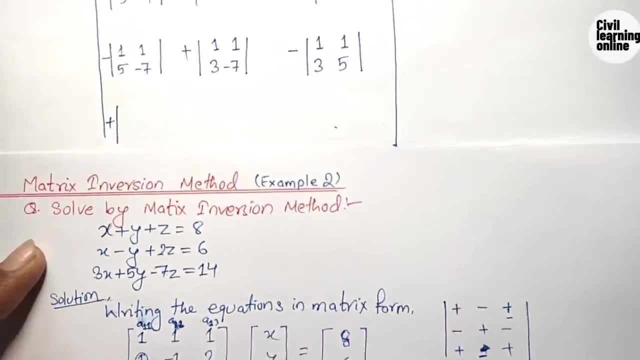 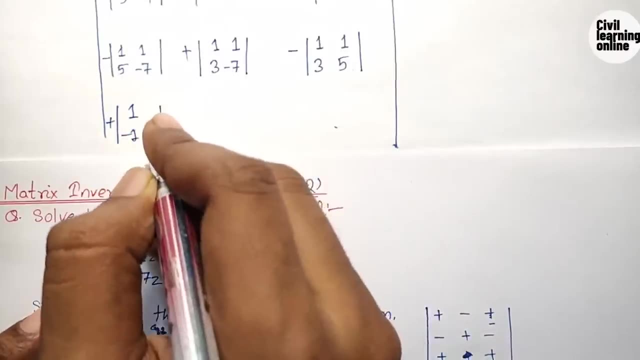 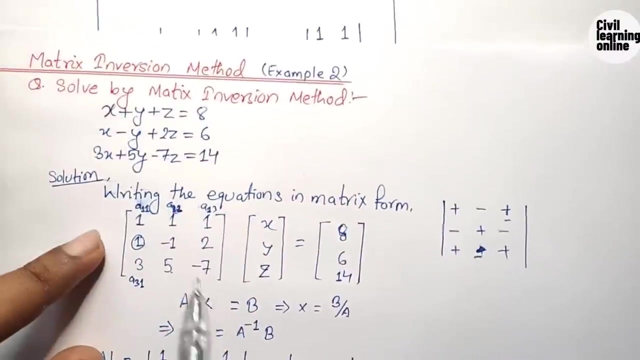 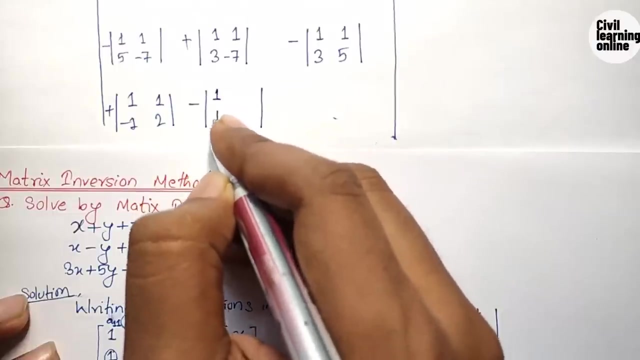 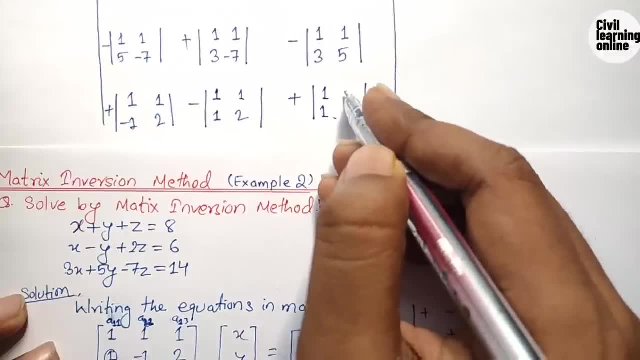 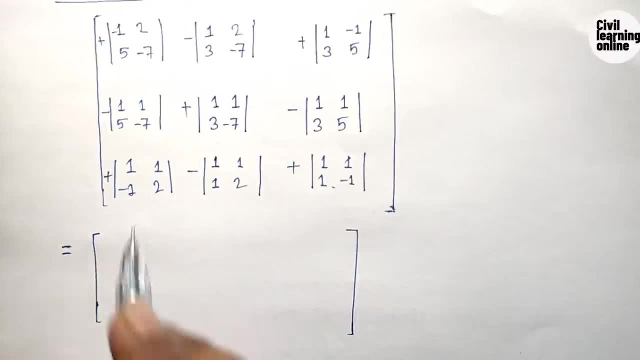 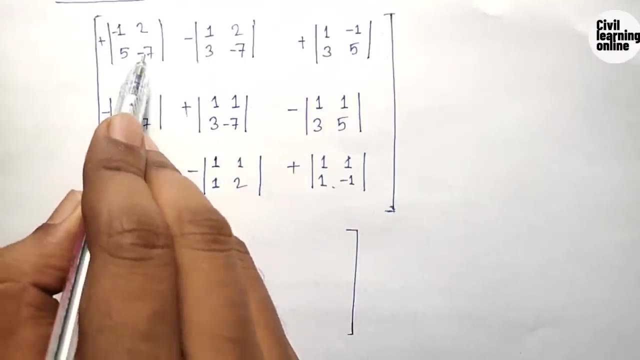 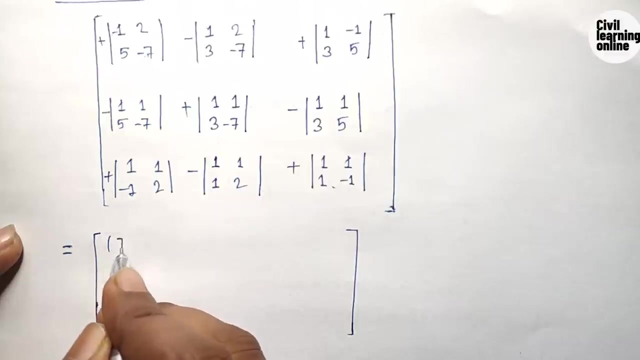 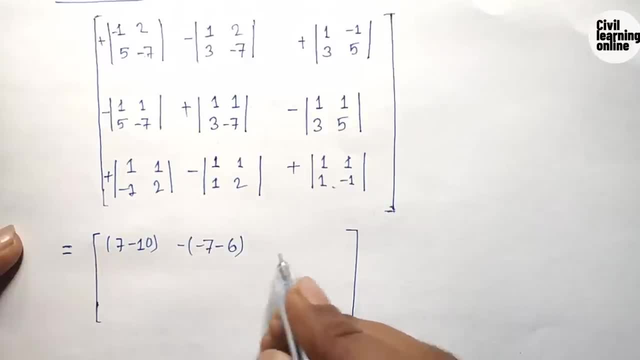 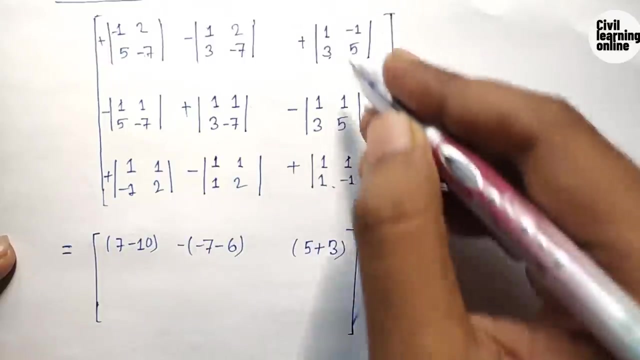 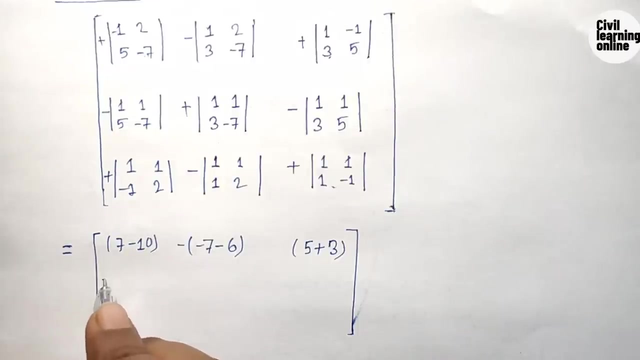 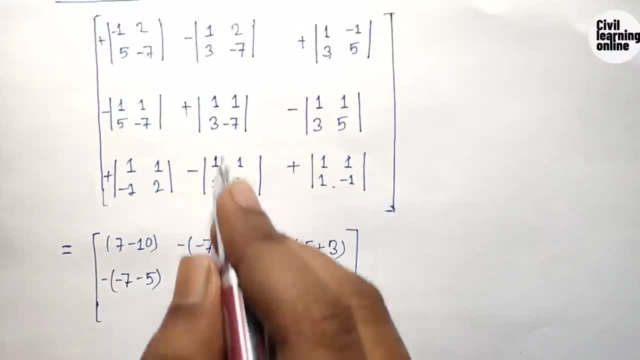 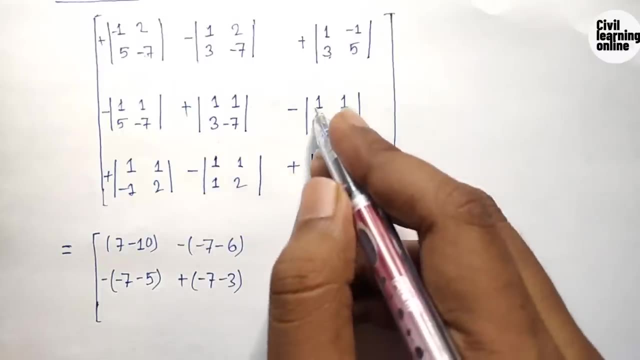 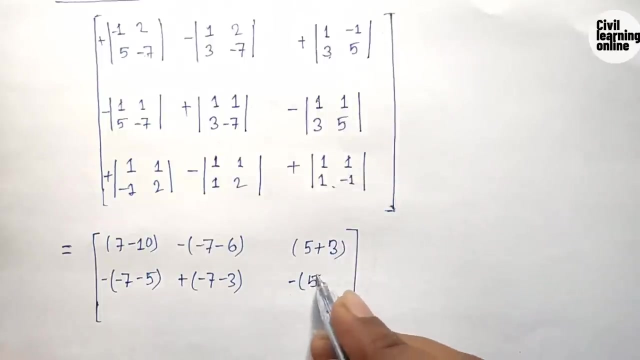 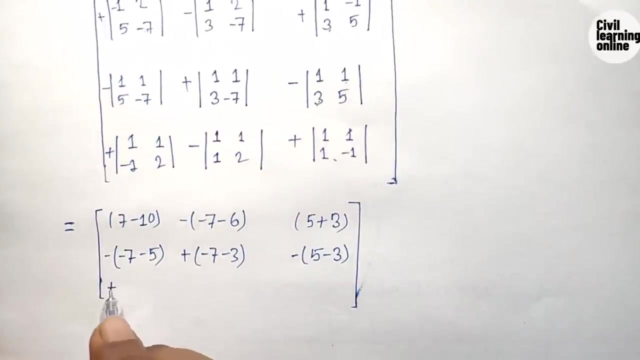 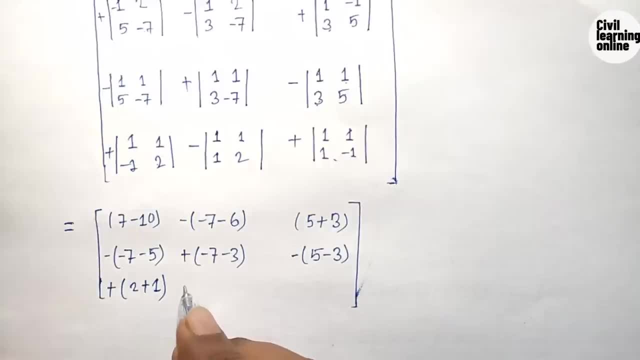 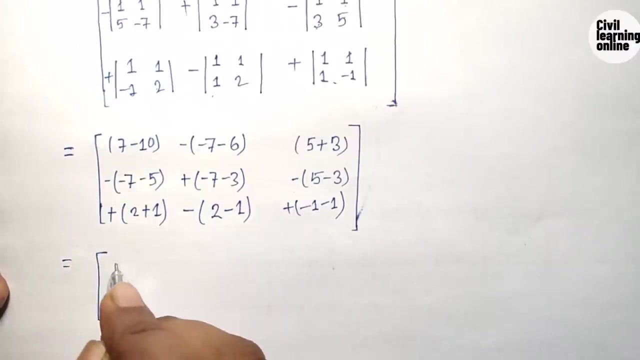 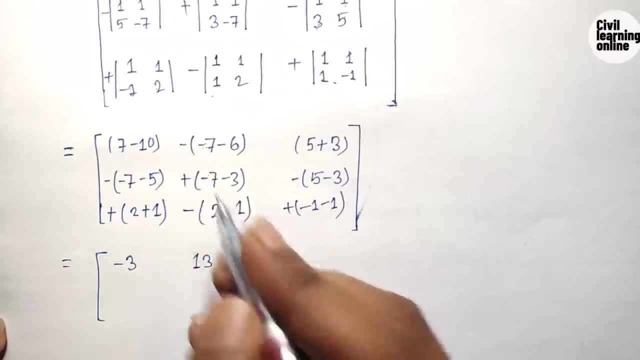 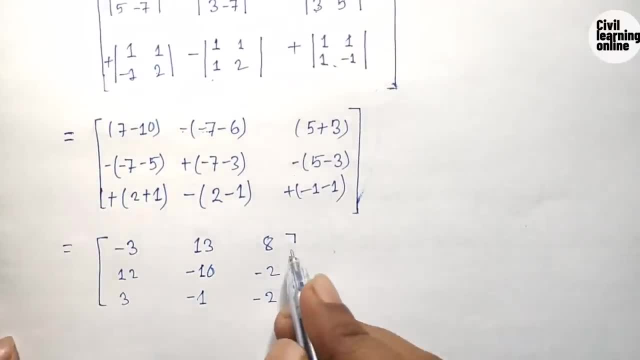 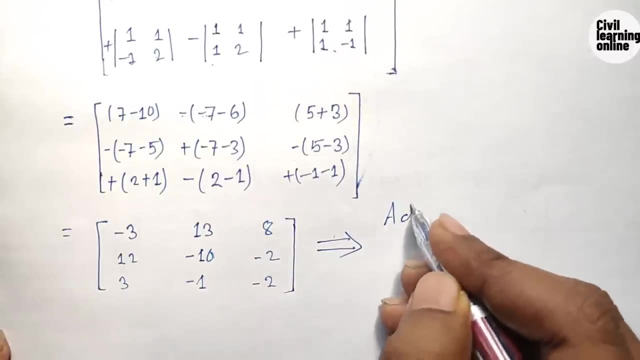 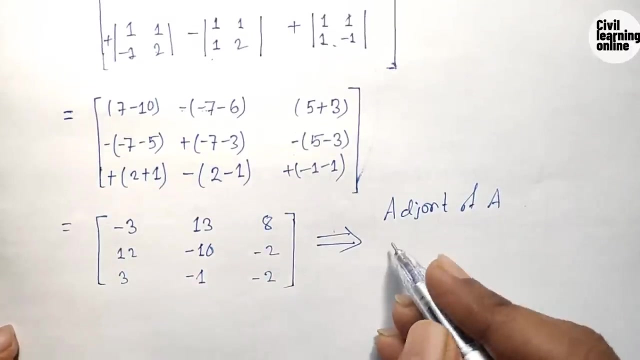 2. now time to calculate the adjoint of the matrix. so adjoint of matrix will be transpose of the cofactor of the matrix. so how to find a transpose of the cofactor? simply copy the diagonal element: minus 3, minus 10, minus 2 and. 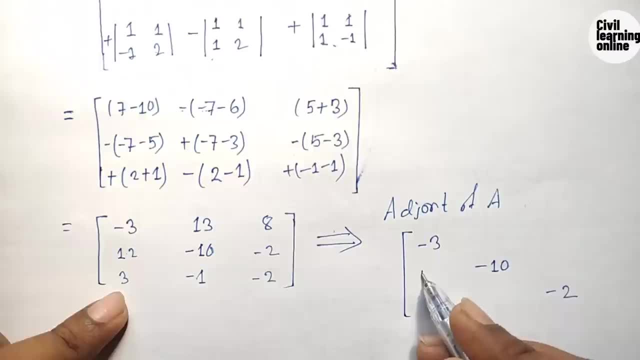 interchange this element, this 13, bring here 13, and write this double here. just interchange the position 3, bring here and 8 here. so 8 and 3. interchange these two, so minus 2 and minus 1. now, after this step, we need to find the inverse of. 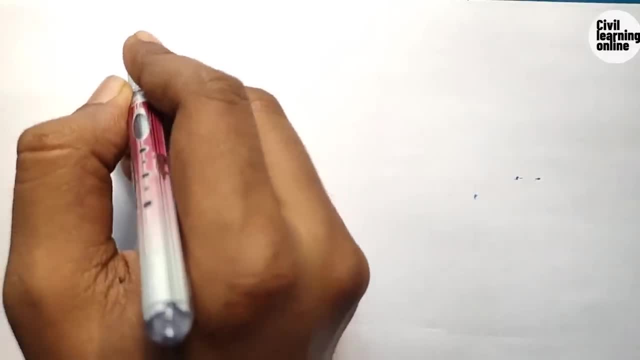 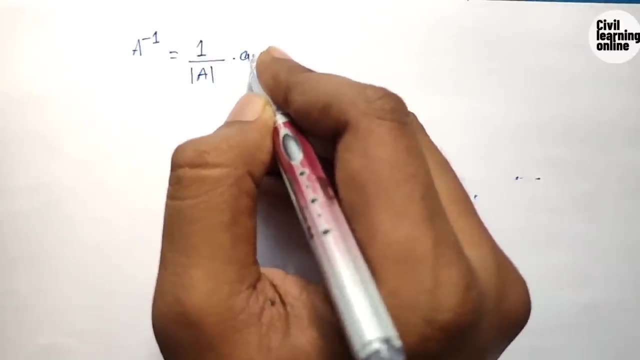 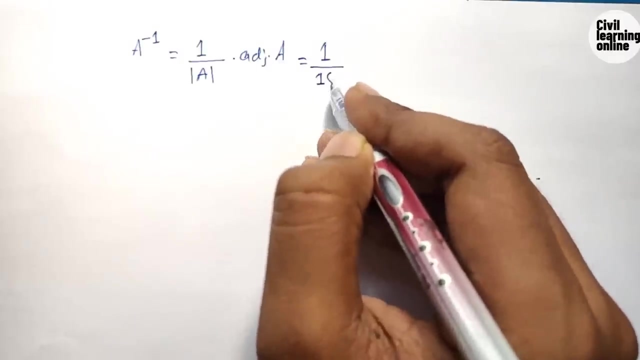 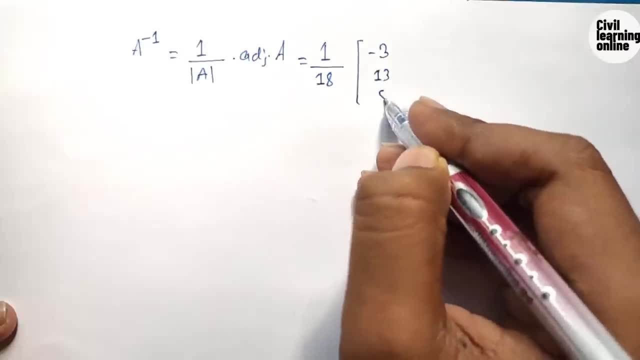 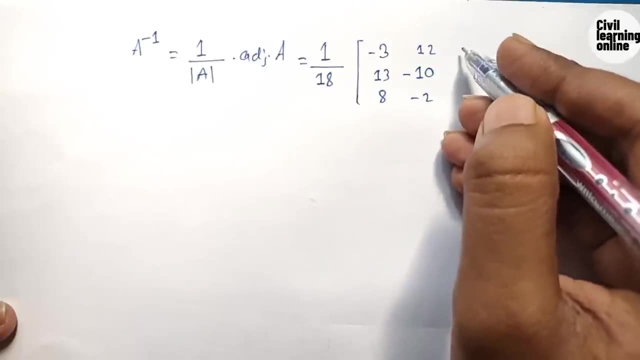 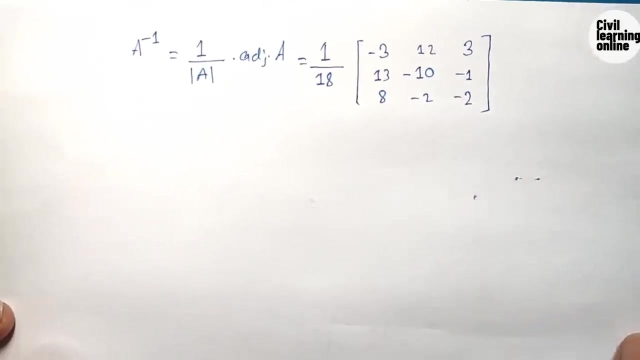 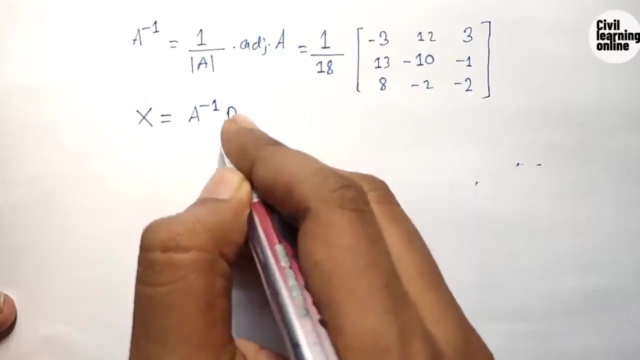 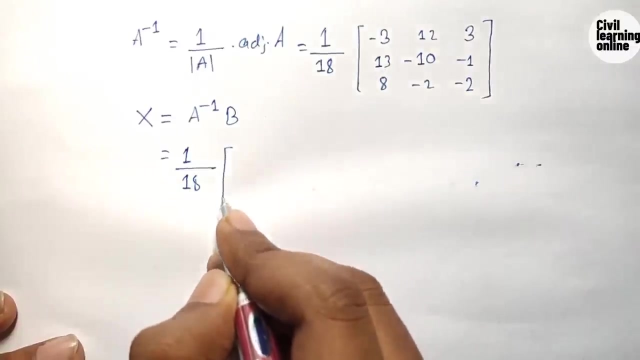 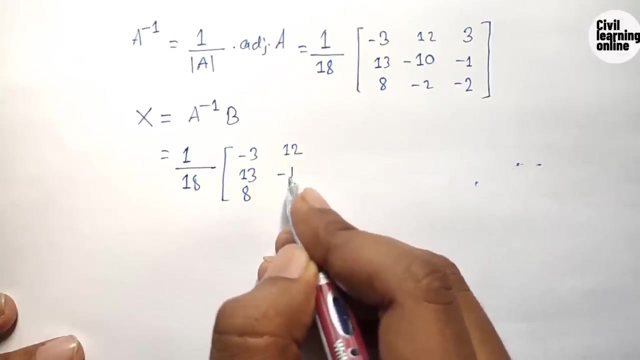 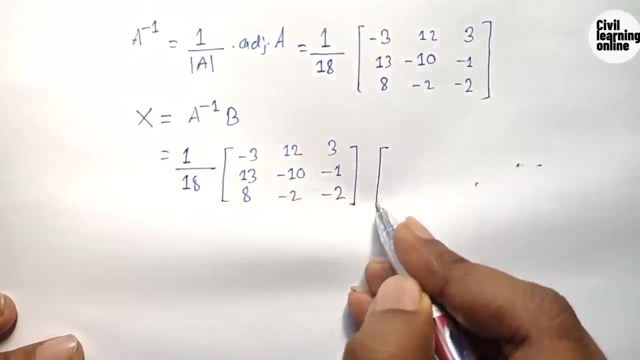 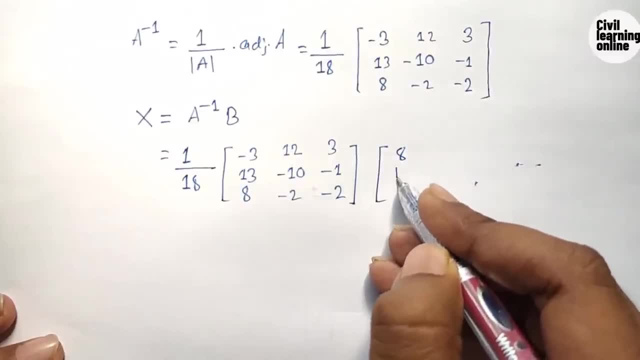 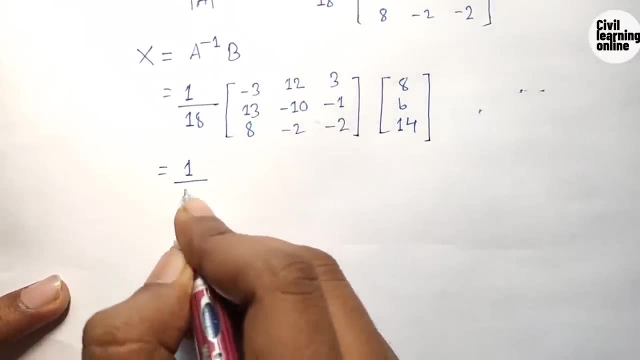 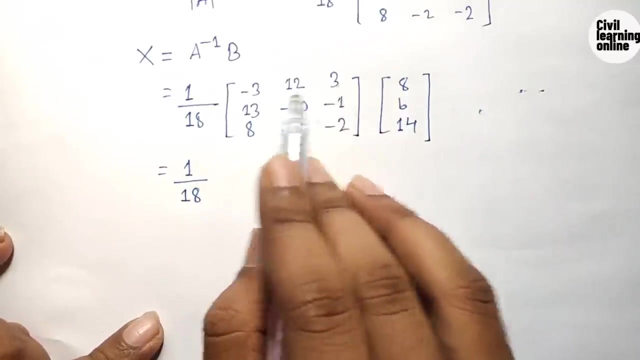 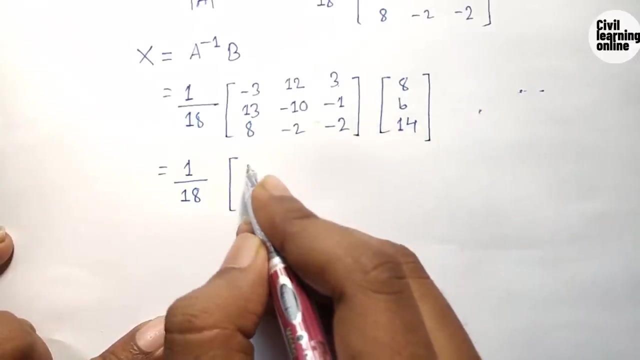 and the element of B are 8, 6 and 14. now, guys, what we need to do is just rewrite the determinant and multiply the element of this first row with the element of this column. so minus 3 times 8 will be equals to minus 24, double times 6 will. 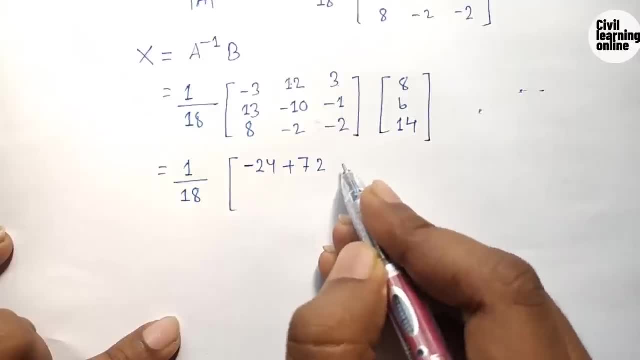 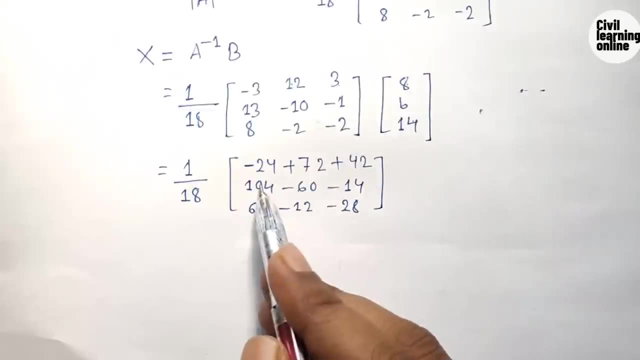 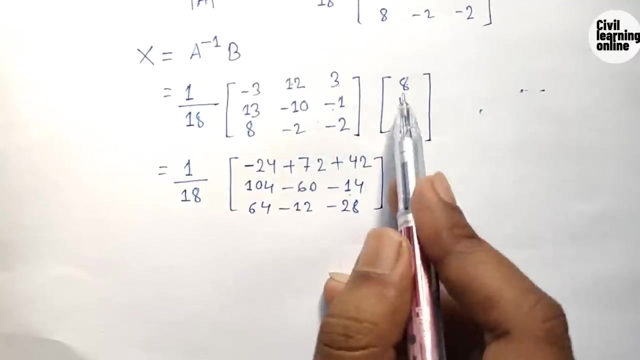 be equals to positive 72 and 14 times 3, 42. similarly, 13 times 8 will be equals to 104 and minus 10: 6. 10 times 6, will be 60. minus 14 it, 8 times it will be 64. 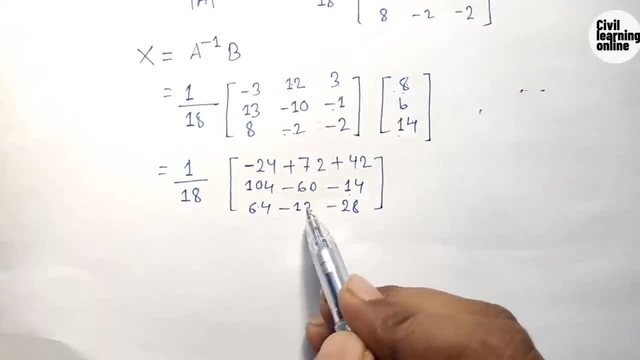 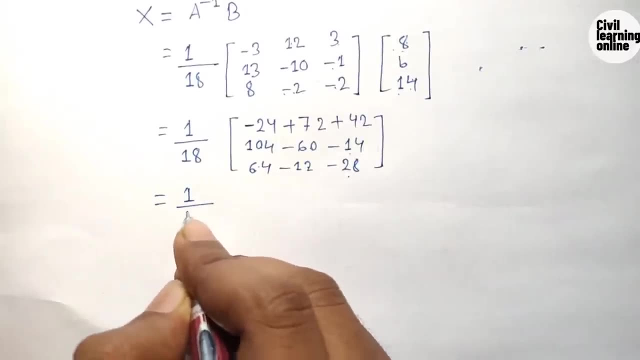 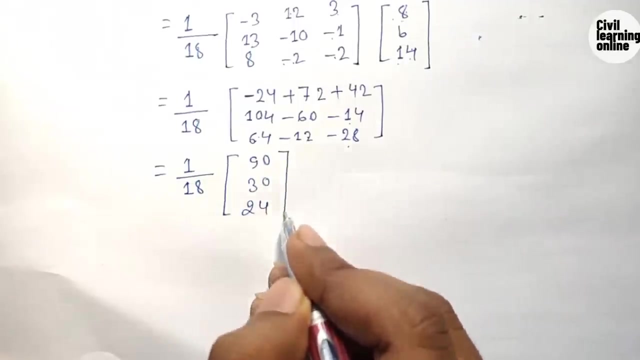 minus 2 times 6 will be equals to minus 2. well, minus 2 times 14 will be equals to minus 28. now, at this, we will have 1 by 18 times 90, 30, 24. now divide these terms with 18, we will get the value of X. 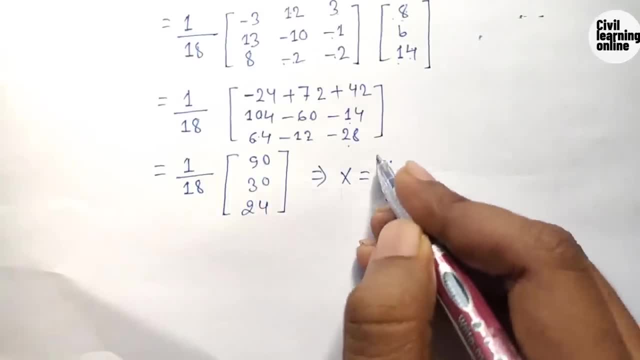 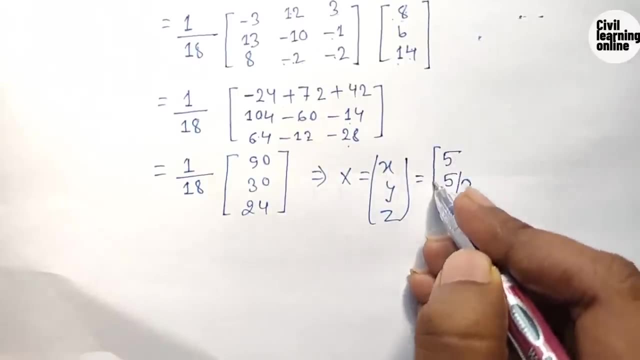 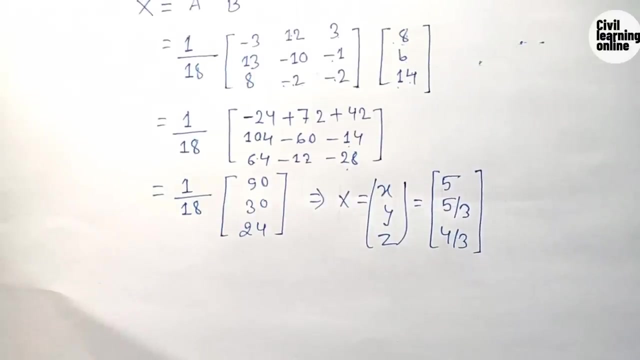 equals to X, Y, Z equals to 5, 5 by 3 and 4 by 3. so, guys, this is the final answer and we have solved this system of linear equation using the matrix inversion method, and I will see you in the next video. Thank you for watching. 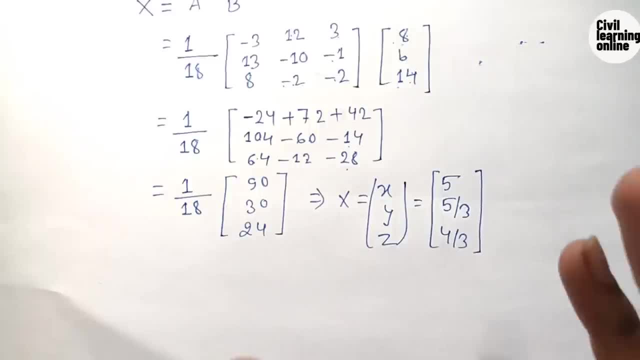 I hope you enjoyed this second example on the matrix inversion method. want to have more videos in the future? then do subscribe to this channel- press the bell icon also- and to share this video with your friends, and I have kept my email in the description as well as in the about section of my channel. you can 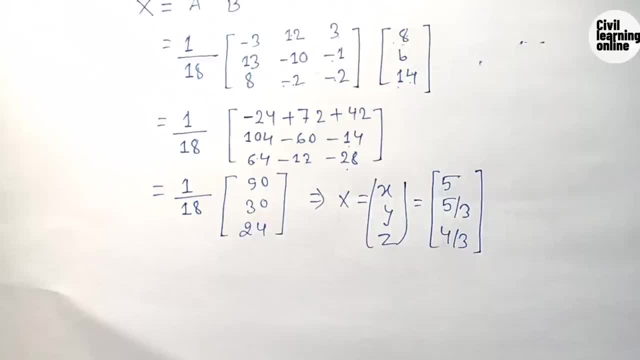 have access the email from there and if you have any kind of query or problem problem, then do write me on the email and we will try my best possible way to reply to your queries in the short period of time and till then, stay safe and take care of yourself. see you in the next video. bye, bye.